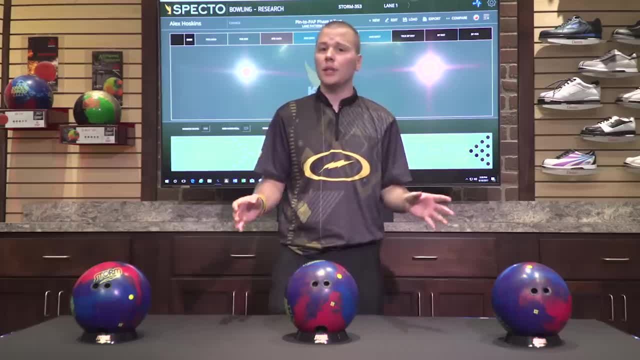 On this table. you see some different falls on the tables. Each phase two bowling ball has a different pin to PAP distance. On the left here we have a one-and-a-half-inch PAP distance. In the middle we have a three-and-a-half inch pin to PAP distance And on the right we have a seven-inch. 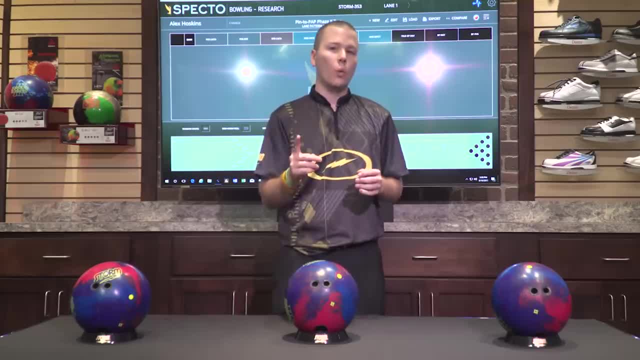 Now on the side note, the other two measurements in Storm's PAP difference And on the Smith and inches, the pin buffer on all three bowling balls one inch. so let's take a look at some graphics and see what's going on when we change that pin to PAP distance on the inside of the bowling ball. 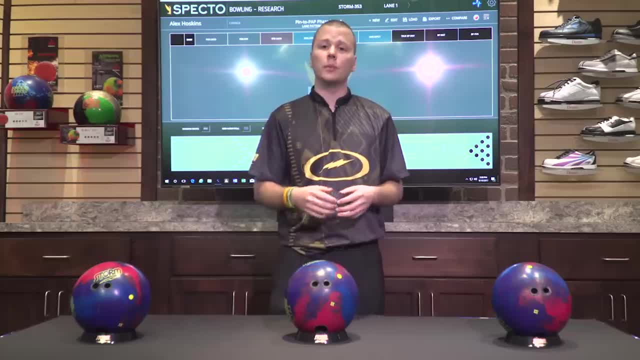 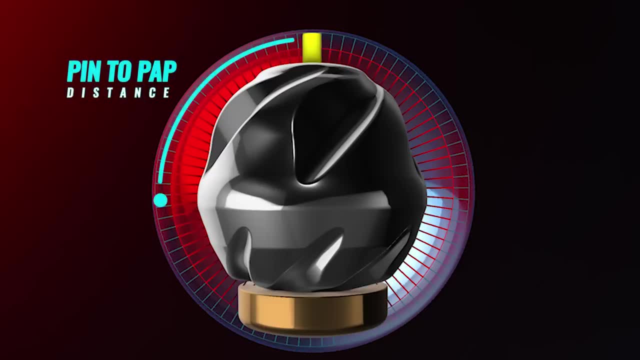 and later we'll see how that translates into ball motion as we throw these balls down the lane. let's take a look. here we have the velocity core that is found inside the phase two. the pin to PAP distance is going to control the amount of flare this velocity core creates. 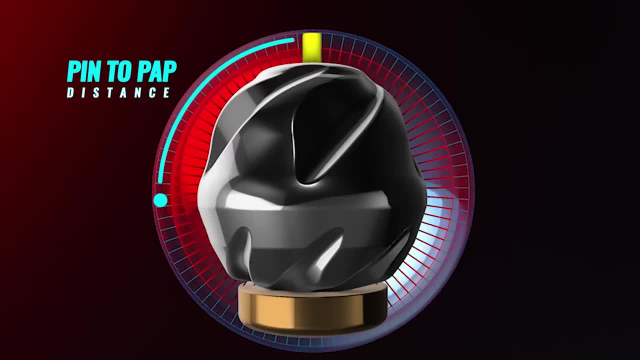 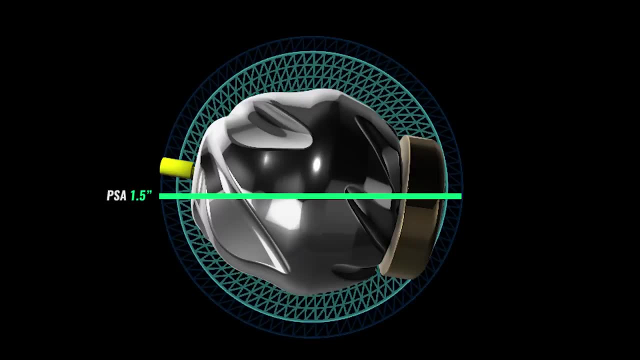 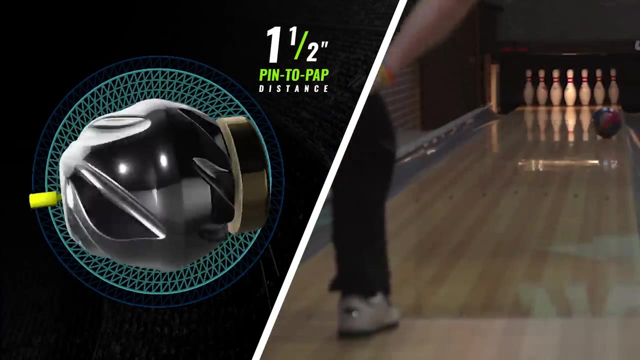 changes in the pin to PAP distance will position the core at different angles at the moment of release. let's position the core with a one and a half inch pin to PAP distance and send it into rotation. you'll see that this lays the core down on its side and the rotation is fairly stable. 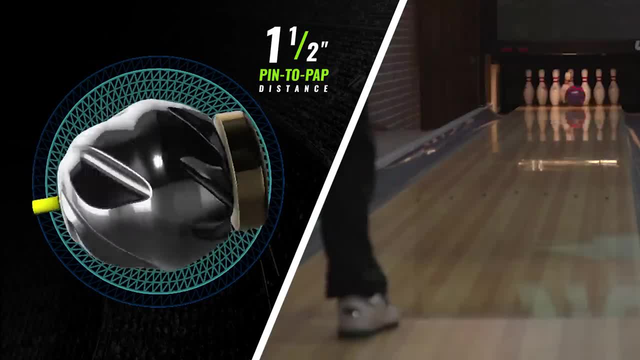 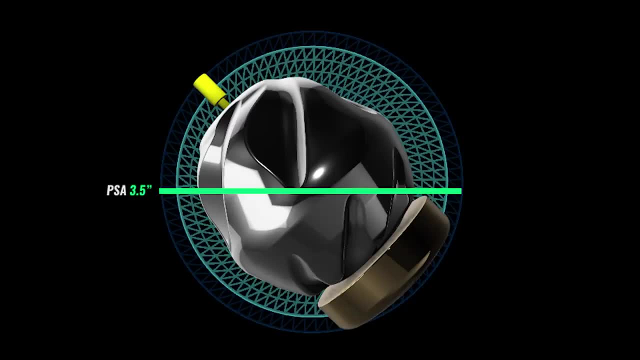 this will result in less overall flare and a smooth motion down the lane. now let's position the core with a three and a half inch pin to PAP distance and send it into rotation. you'll now see how much more unstable the rotation is. this is because the core is sitting. 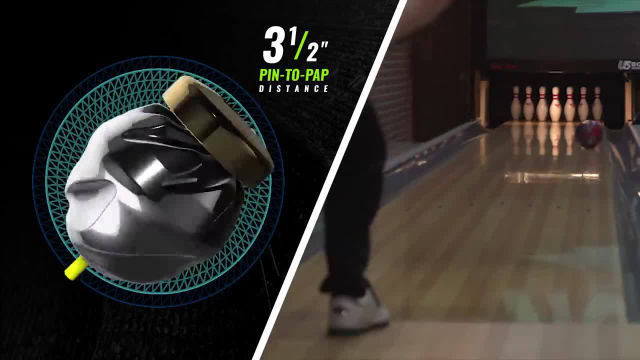 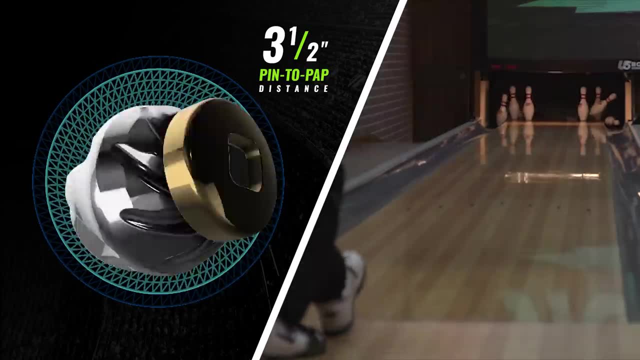 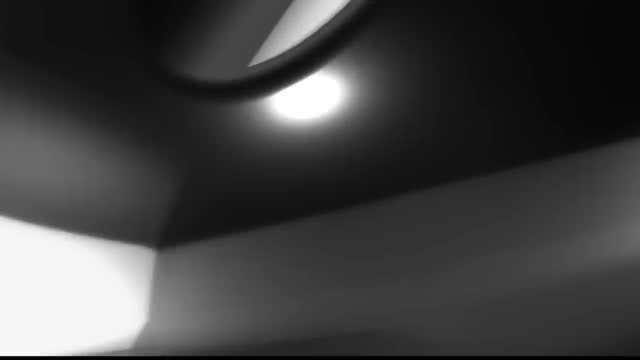 at nearly a 45 degree angle on the inside of the bowling ball. upon release it is very unstable and needs to migrate significantly to achieve a stable position. this will result in more overall flare and much more motion both front to back and left to right. finally, let's position the core with a six inch pin to PAP distance and send it into rotation. 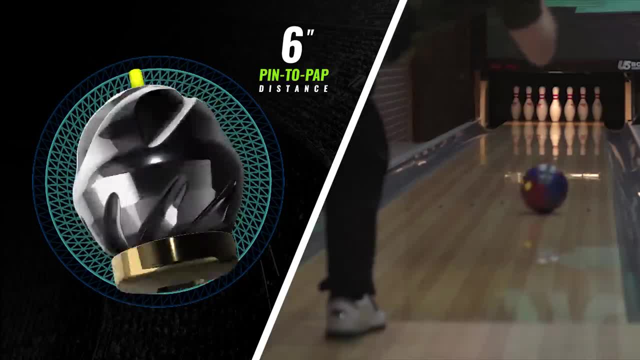 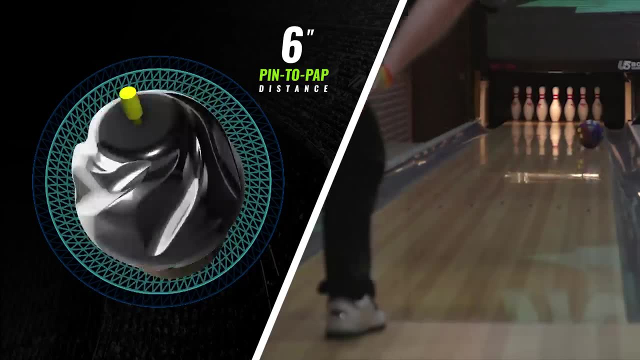 you'll see that this nearly stands the core completely up at the moment of release. it is not going to have to migrate very far to achieve a stable position. this will result in less overall flare, a much straighter path through the front part of the lane and more motion at the 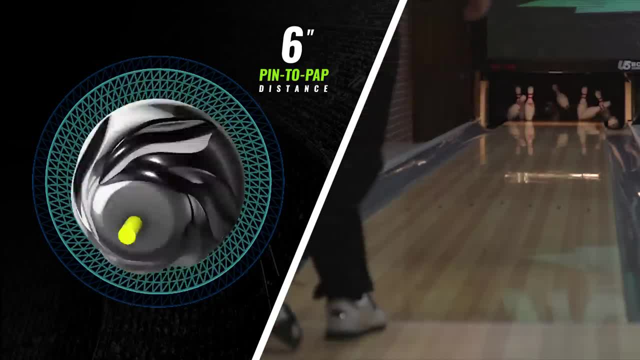 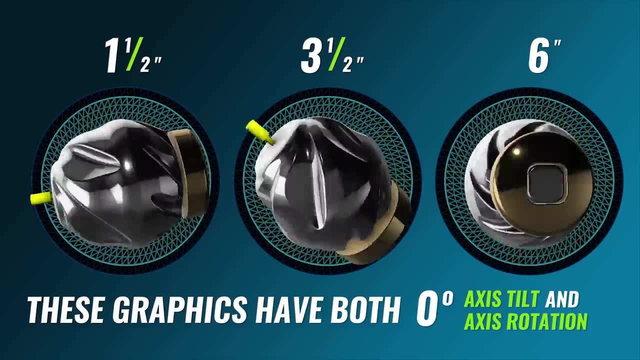 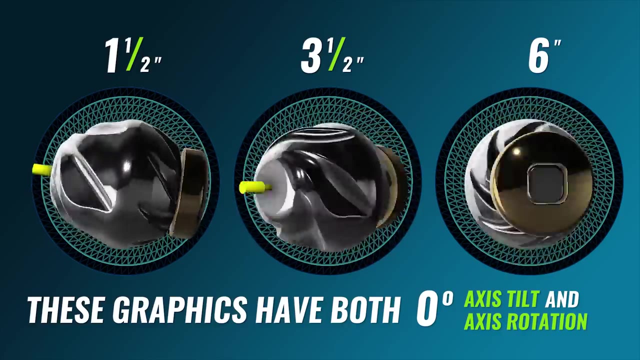 end of the pattern if there is enough friction in the back part of the lane. keep in mind these graphics have both zero degrees of both axis tilt and axis rotation. we are just using these as a reference to see the angle in which the core is oriented at the moment of release, with different 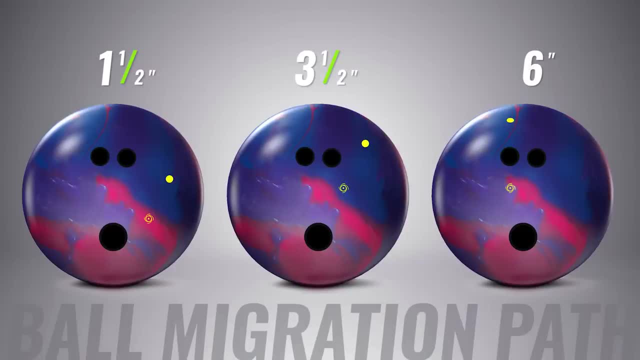 pin to PAP distances. we have put some contrasting markers on each of these bowling balls to help you see how the migration is occurring as we watch these balls go down the lane. the first marker was placed on the initial positive axis point. the second marker was placed exactly two inches away. 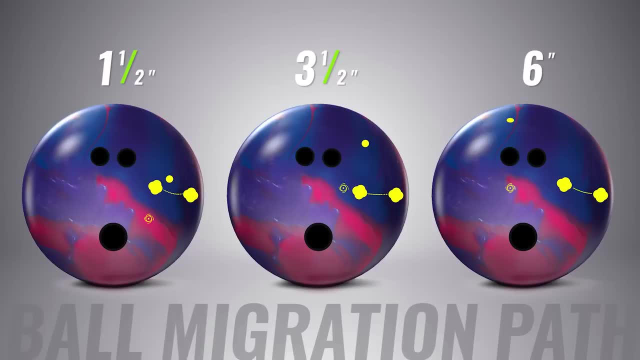 from the positive axis point along the migration path so we can see how quickly the migration over this point. keep in mind this second marker doesn't necessarily represent the final axis the ball achieves when it is rolling in the six inch pin to PAP distance picture it is the final axis. 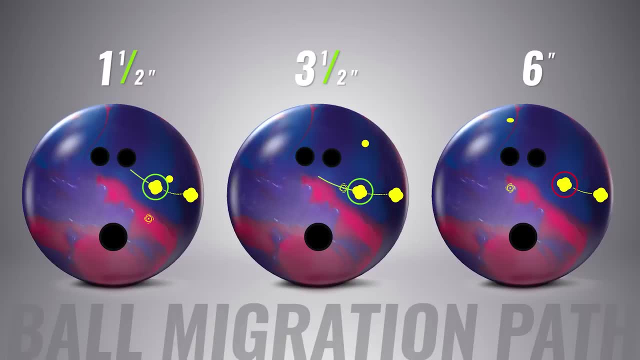 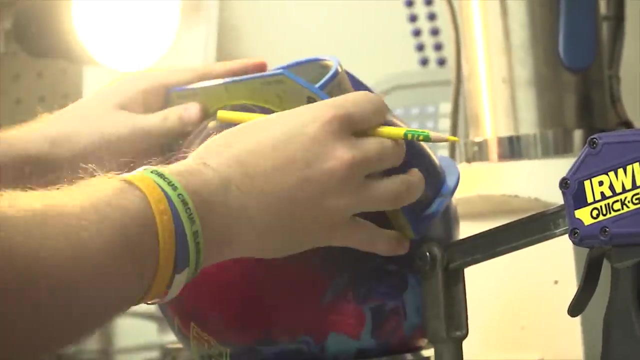 because the ball only has two inches of total flare. we are just using these markers as a visual aid to help us see how unstable the ball is and how quickly it is migrating as it goes down the lane. this first video compares the one and a half inch phase two to the three and a half inch phase two. 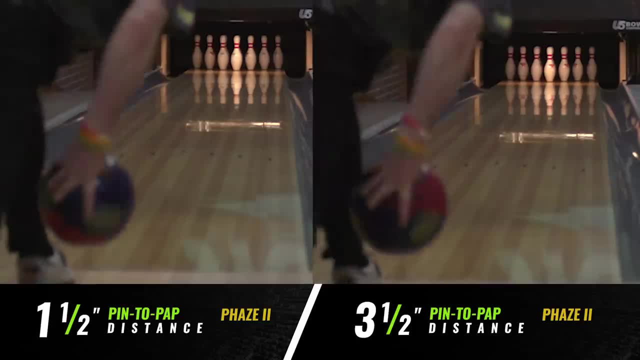 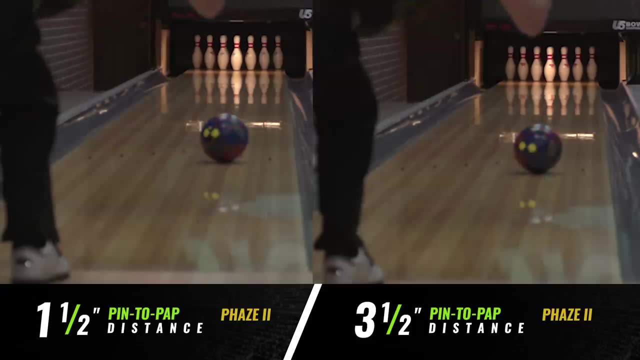 the first difference you'll notice is how quickly the migration reaches the second colored marker on each of the balls. take a look at the three and a half inch phase two. on the right, the second colored marker lines up at the arrows. now take a look at the one and a half inch phase. 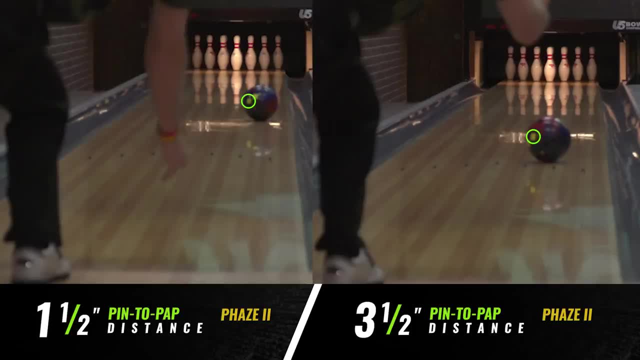 two on the left. the second colored marker lines up at about 30 feet down the lane. this is a significant difference and shows you how much stronger the three and a half 2 is front to back, Since the 1.5-inch Phase 2 is in a more stable position upon release. 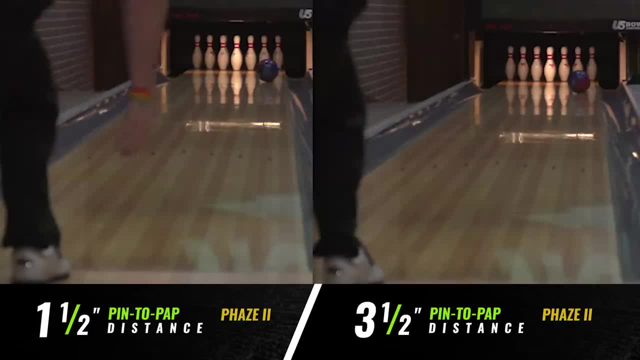 it creates a much smoother, predictable motion throughout the entire lane As the balls enter the pins. the 3.5-inch Phase 2 finishes higher because it is much stronger throughout the entire lane than the 1.5-inch Phase 2.. This will generally be better for speed-dominant. 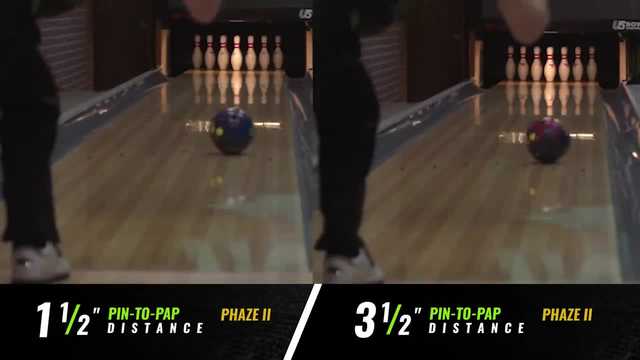 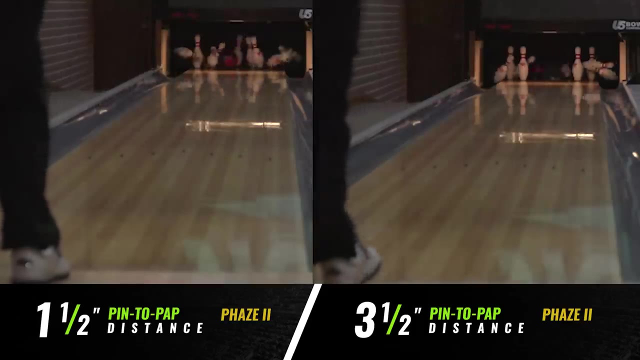 players because the core is in such an unstable position upon release that it creates a massive amount of flare. If you're a player with higher ball speed looking for more overall hook, try some stronger pin-to-PAP distances. Keep in mind there can always be exceptions. 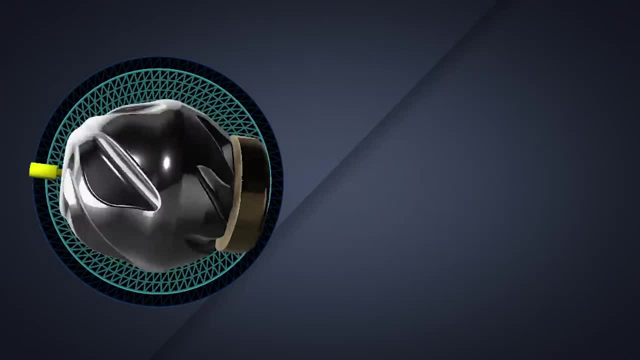 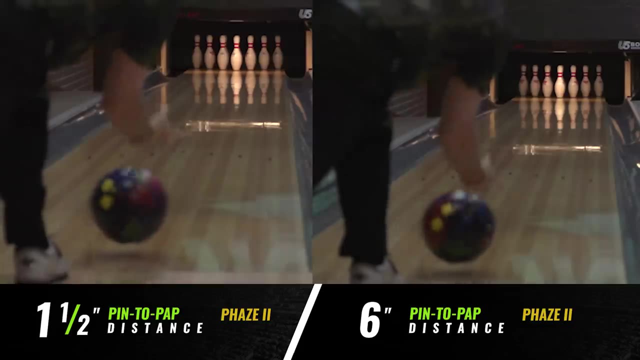 but this is a good rule of thumb. This time we're comparing the 1.5-inch Phase 2 to the 6-inch Phase 2.. The first difference you'll notice is how long it takes for the 6-inch Phase 2 on the right to get to the second colored marker. It stays on its initial axis. 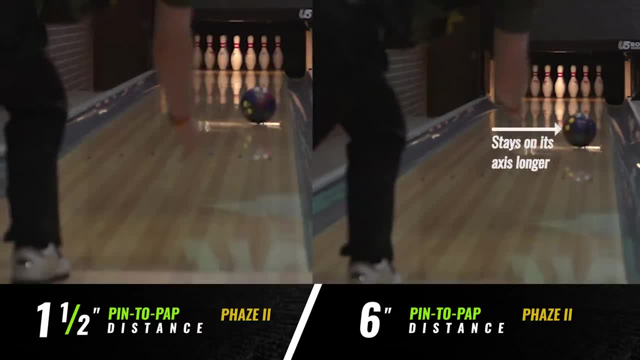 much longer because the ball is in a more stable position upon release. and the ball is in a more stable position about the high-RG axis. The second colored marker doesn't line up until just before the ball enters the pins, As we saw in the previous video. the 1.5-inch 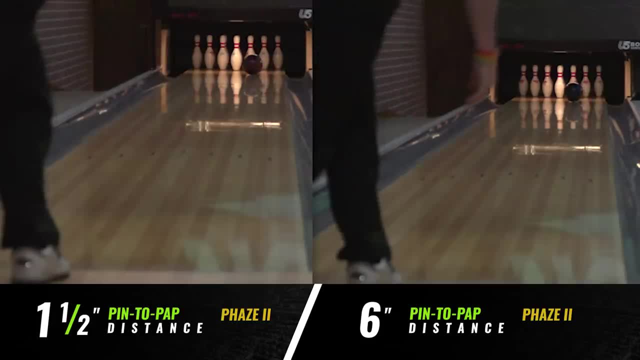 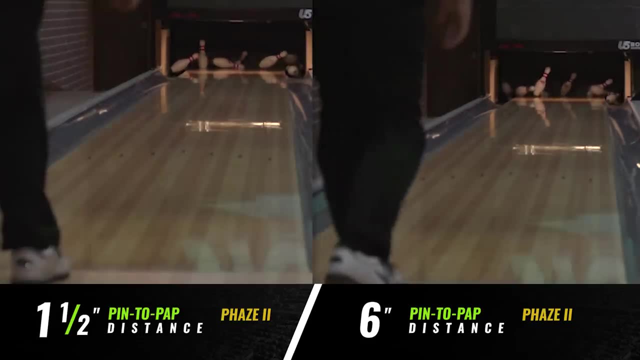 Phase 2 on the left lines up at about 30 feet down the lane. Take a look at how each ball creates a different shape as they go down the lane, even though they are utilizing a similar amount of flare. This shows you how important it is to utilize. 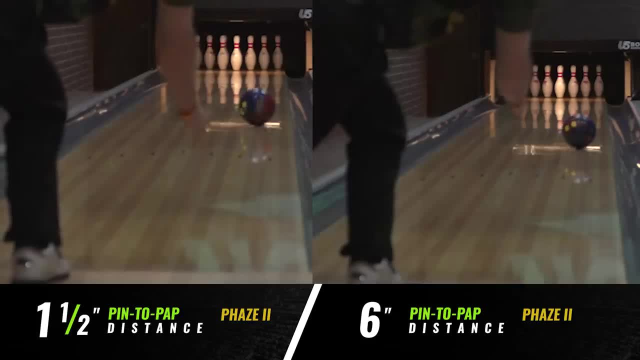 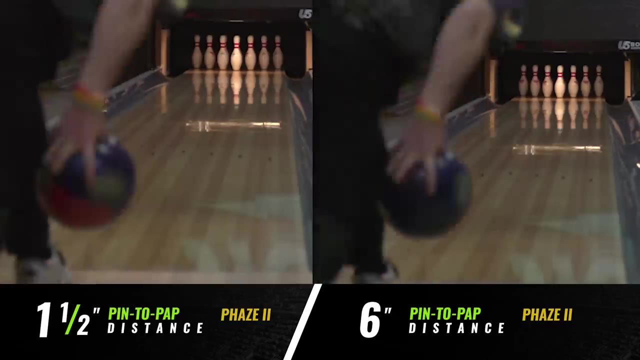 both low and high-RG layouts in your arsenal. Shorter pin-to-PAP distances, such as the 1.5-inch Phase 2 on the left, can be useful when the pattern is extremely short or you're looking for some control off the end of the pattern. They can also be good for rev-dominant. 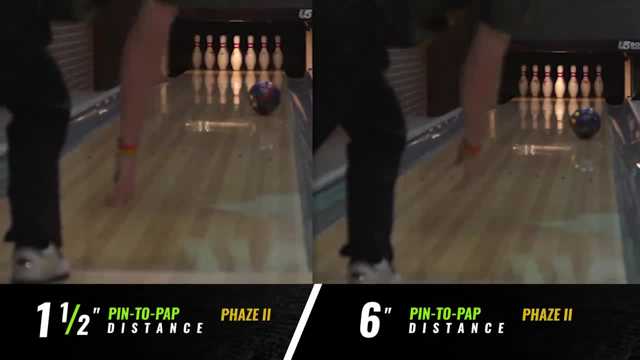 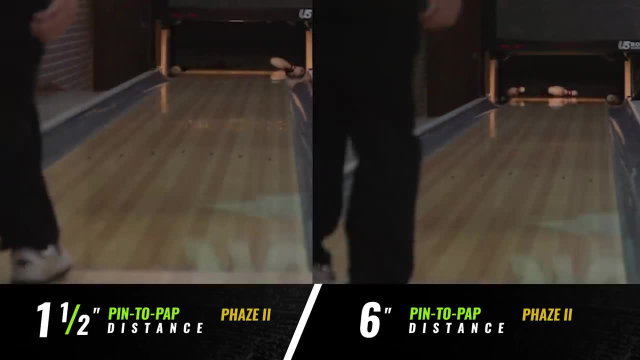 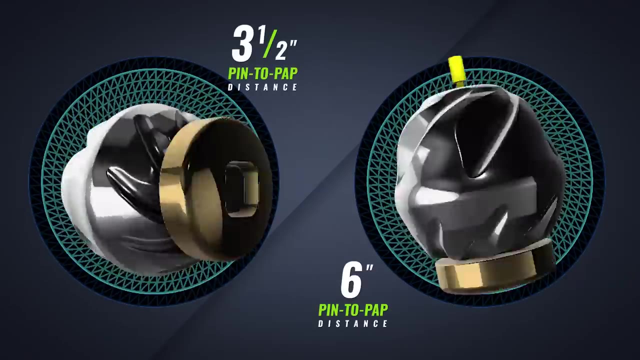 players looking to keep their ball under control when there is a significant amount of friction in the back part of the lane. Keep in mind there can always be exceptions, but this is a good rule of thumb. This final video compares the 3.5-inch Phase 2 to the 6-inch Phase 2.. These two have extreme 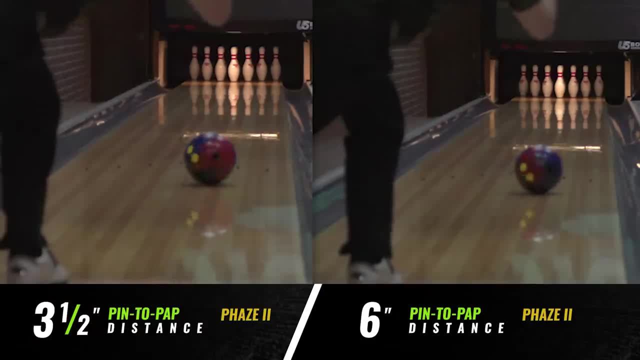 differences. On the 3.5-inch Phase 2 on the left, the second colored marker lines up at the arrows. Take a look at the 6-inch Phase 2 on the right, in the same place. It still hasn't even migrated off its initial axis yet. It is much cleaner through the front. 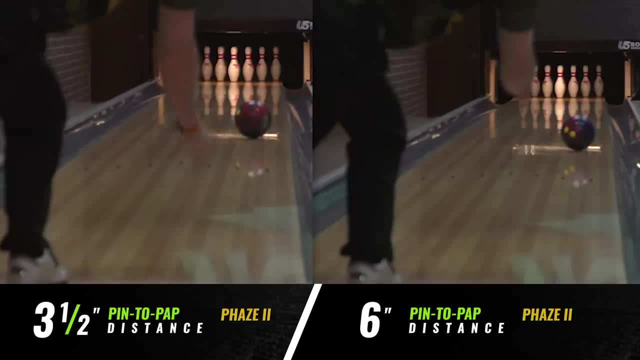 part of the lane because less energy is used through the first 15 feet of the lane. This shows you why longer pin-to-PAP distances are important. Imagine trying to get the 3.5-inch Phase 2 through the front part of the lane at the 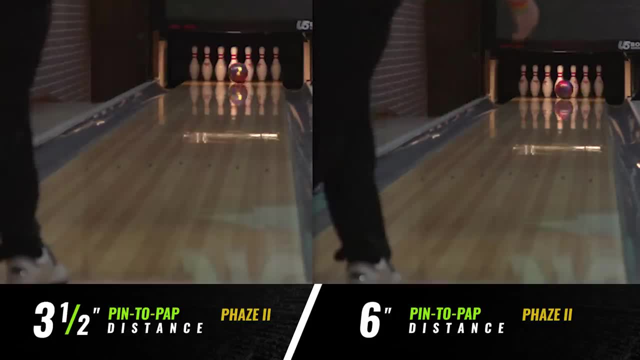 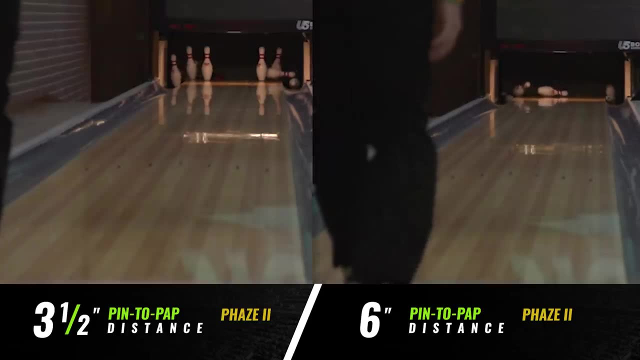 end of the night of league. It would be extremely difficult to get the ball through the pins with enough energy to strike when a majority of the energy is being used in the front part of the lane. The 6-inch Phase 2 will get you through the friction cleaner and save more.